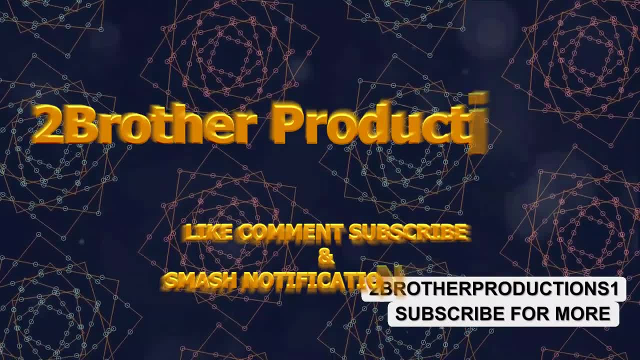 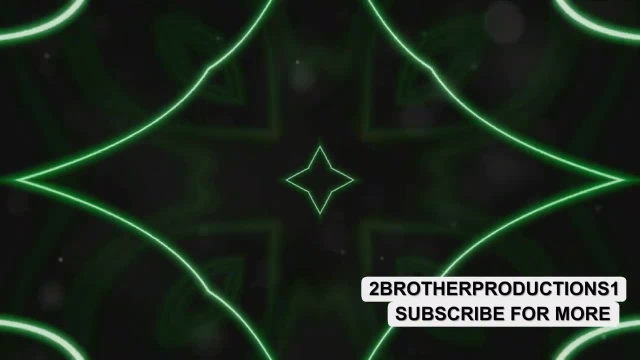 non-Euclidean geometry presents an alternate reality where straight lines aren't the shortest distance between two points and parallel lines may intersect. It's as if the rules of the game have been rewritten. Now imagine a space that's curved like the surface of a sphere or 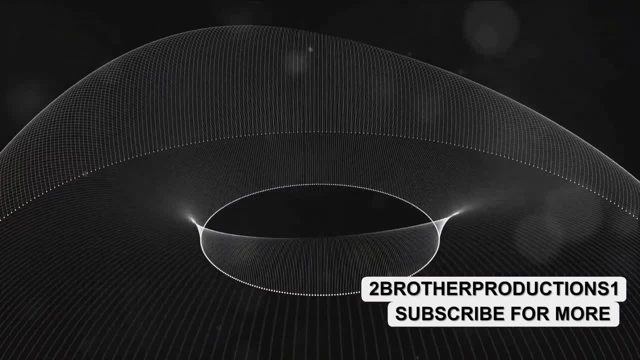 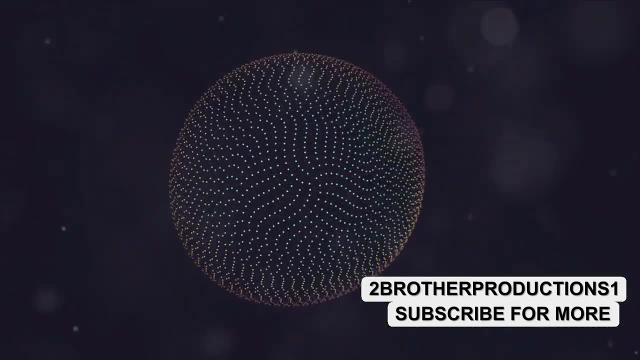 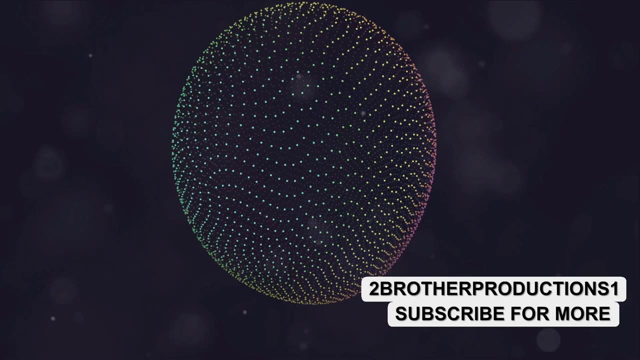 the shape of a saddle. This is the essence of non-Euclidean geometry, which branches into two primary forms: hyperbolic and elliptic. Hyperbolic geometry, like a saddle's surface, allows for lines to diverge, while elliptic geometry, similar to a sphere's surface, makes parallel lines meet. 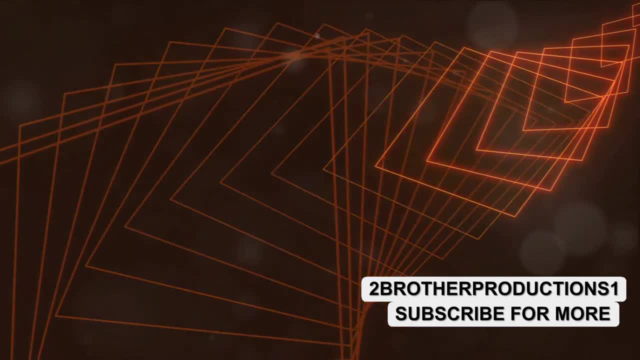 So, in a nutshell, non-Euclidean geometry breaks down In a nutshell, non-Euclidean geometry breaks down. In a nutshell, non-Euclidean geometry breaks the flat rules and bends our understanding of space. Quite the enigma, isn't it? Why should we? 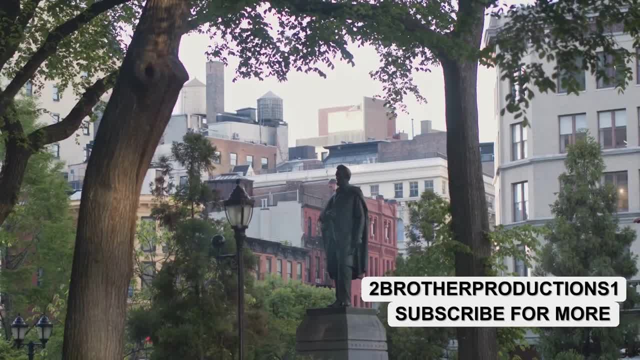 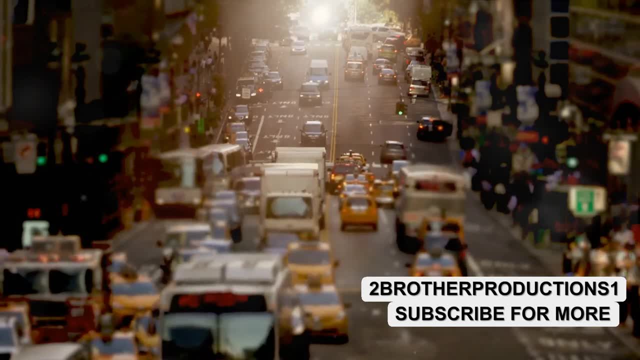 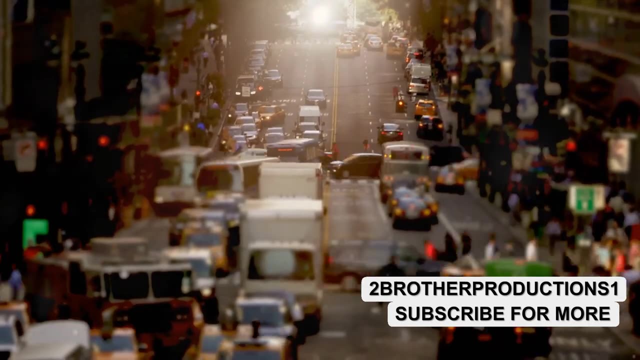 care about non-Euclidean geometry, you may ask? Well, its impact is far greater than what one might initially perceive. This form of geometry, which may seem abstract and obscure, is in fact, fundamental to our understanding of the universe. Imagine a world where Albert Einstein never used. 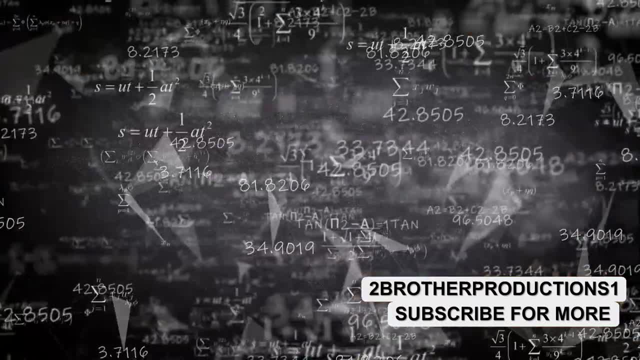 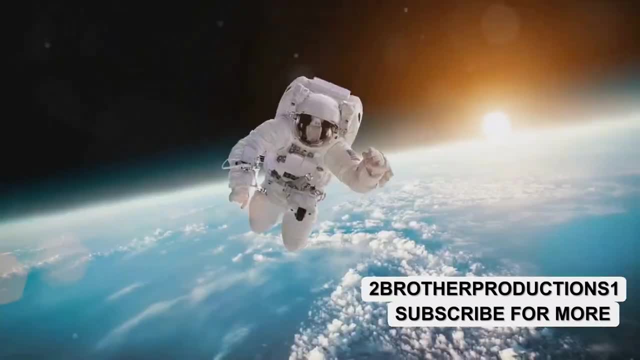 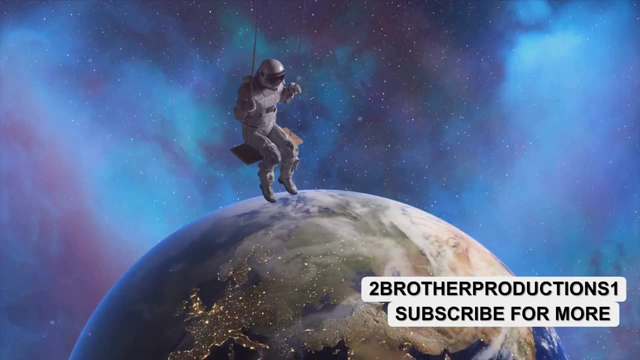 non-Euclidean geometry to develop his theory of relativity. Without this mathematical tool, our understanding of gravity, space and time would be vastly different. Einstein's groundbreaking work has forever altered the way we perceive the universe and our place within it. But the 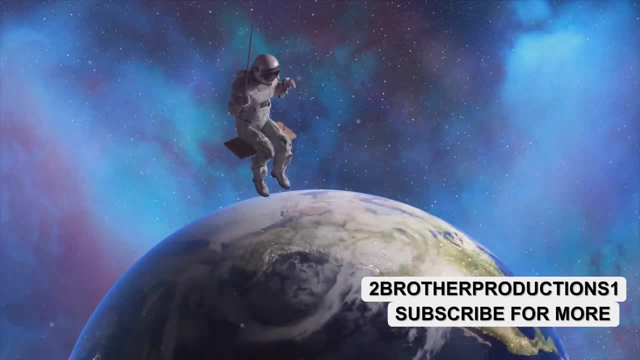 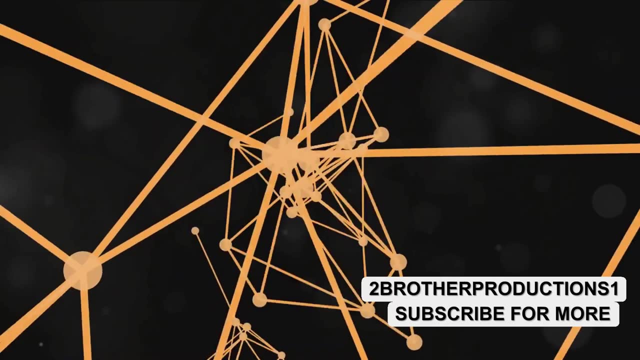 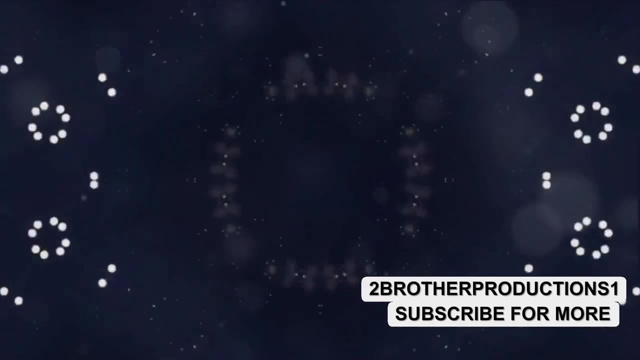 influence of non-Euclidean geometry extends beyond theoretical physics. It's also deeply embedded in our everyday technology. For instance, the global positioning system, or GPS, relies on principles of non-Euclidean geometry for accurate navigation. So, while the concepts might seem far removed from 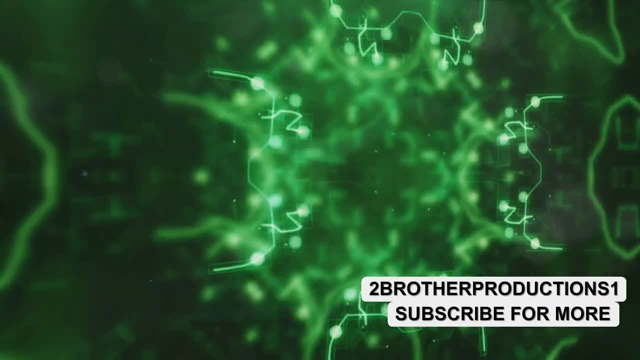 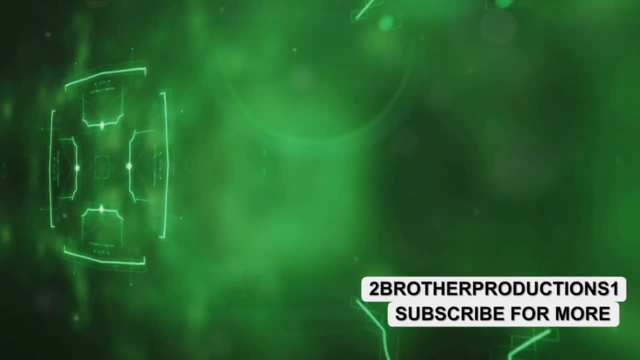 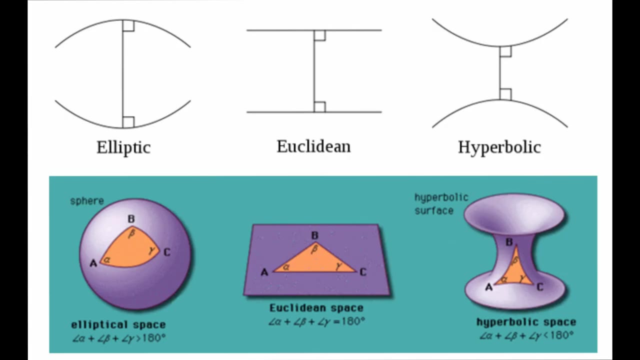 our daily lives. their applications are very much a part of the world we live in. Despite its abstract nature, non-Euclidean geometry has concrete implications that shape our reality. Non-Euclidean geometry- A mind-bending concept, isn't it? We've journeyed through the intriguing landscape of this. 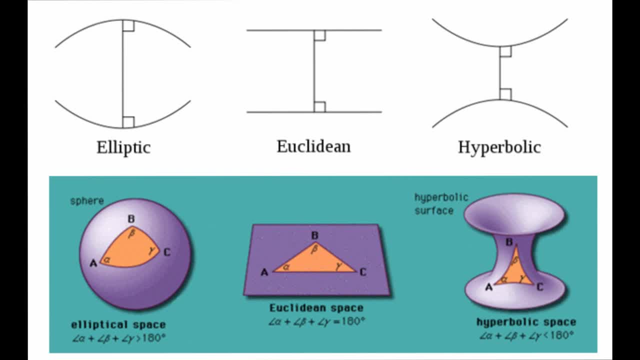 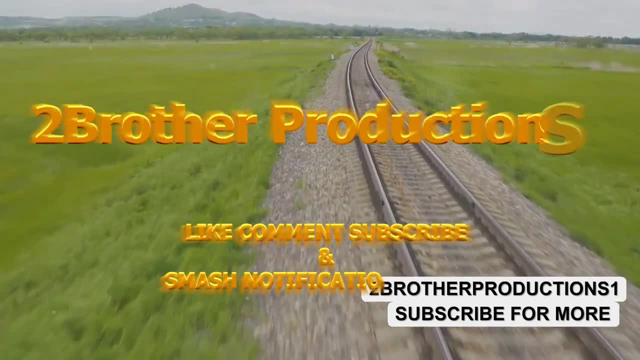 mathematical marvel, challenging our understanding of flat space and straight lines. We've grappled with hyperbolic and elliptic geometries where parallel lines can diverge or converge, defying the Euclidean postulates we once took for granted. We've seen how this abstract concept